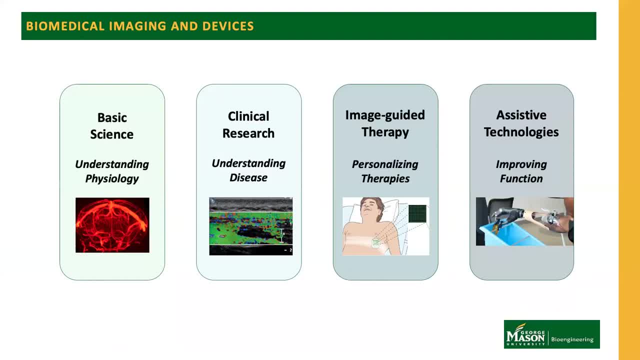 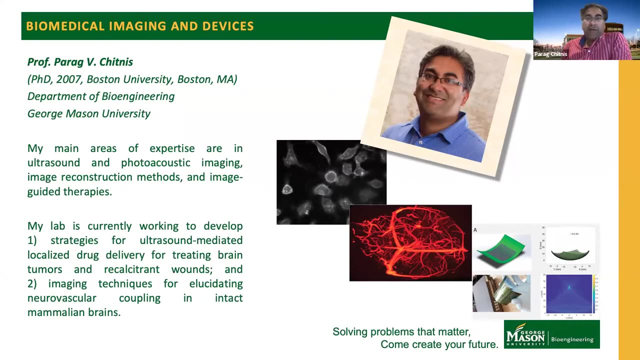 develop image-guided therapeutic strategies for personalized medicine. and developing and evaluating novel assistive techniques, such as prosthetic control systems utilizing wearable imaging sensors to improve function. Hello, my name is Parag Chitnas. I'm an Associate Professor of Bioengineering at George Mason University. 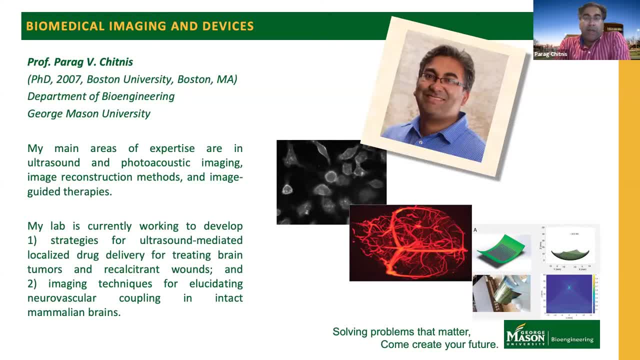 And today I wanted to discuss with you some active projects in our lab. My main areas of expertise are in ultrasound, photoacoustic imaging, image reconstruction and image-guided therapies, And I wanted to cover two projects in my lab today. One involves ultrasound mediated localized drug. 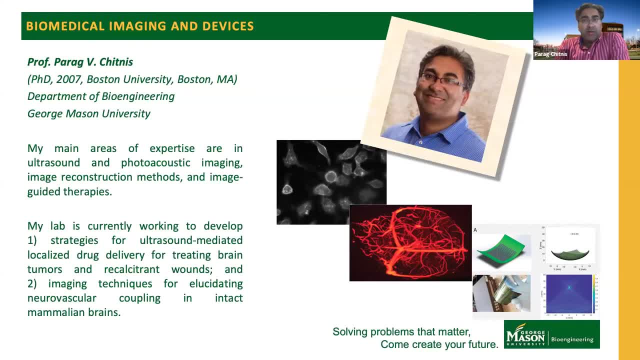 delivery which can be used for treating brain tumors or very difficult to heal wounds. Second is photoacoustic imaging for understanding the brain. Specifically, we're interested in understanding neurovascular coupling. So for the first project, we are developing ultrasound methods for localized drug delivery. 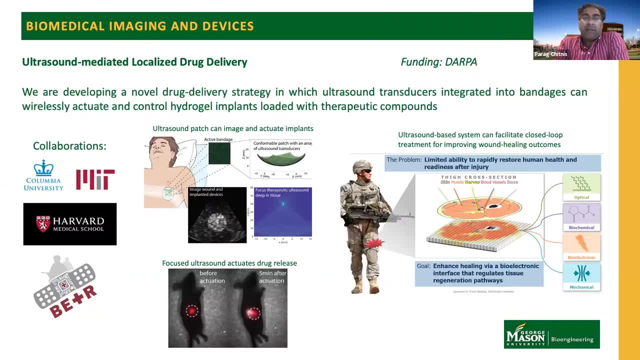 Specifically, we're doing two things. One is developing flexible ultrasound transducers that can be integrated with bandages. Second, we are developing biomaterials, often made from hydrogels, and in addition to that we are developing ultrasonic disruptors, So those ultrasonic 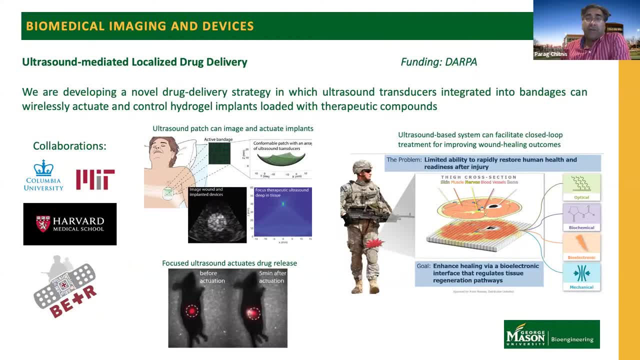 transducers are integrated with therapeutic compounds and can be made responsive to ultrasound. So the ultrasound transducers can then do two things. One, they can image the devices and tissue and help with targeting and keeping monitoring. Second, they can precisely focus ultrasonic energy at the devices and actually release of those therapeutic compounds. 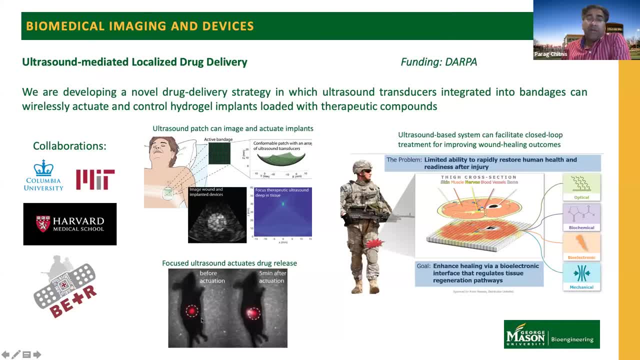 In a previous study we demonstrated the use of NIPAM. hydrogels compound was sequestered nicely within the device before ultrasonic actuation And just five minutes after actuation we can see a nice release of the fluorescent compound from that device. So in this 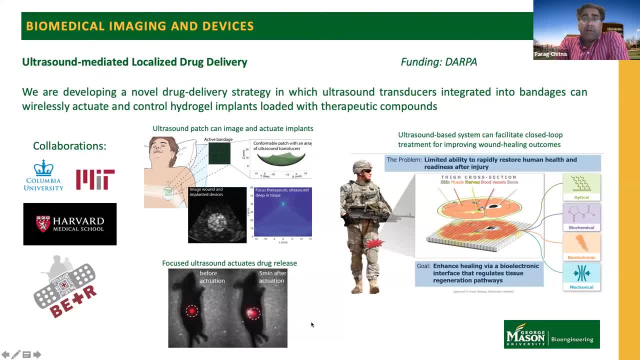 project which is funded by DARPA. we have a consortium of several institutions led by Columbia University, and that includes MIT Harvard Medical Center as well, And we are working actively to use these methods and develop them for treating traumatic injuries suffered by military. 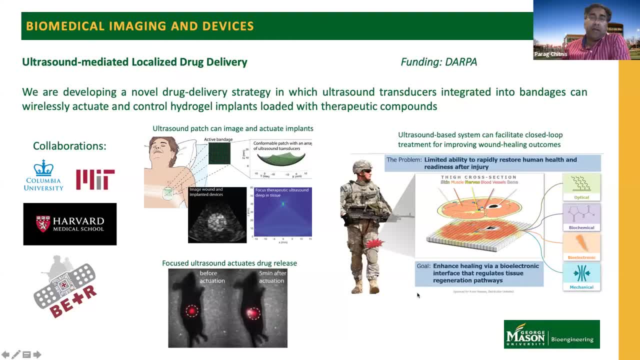 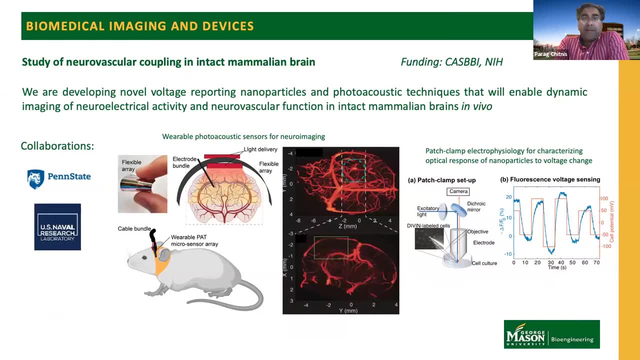 personnel. In another project we're using photoacoustic imaging to better understand brain function. So photoacoustic imaging is a hybrid imaging technique which combines the benefit of light and sound. So optics is sensitive to molecules or function and ultrasound can penetrate. 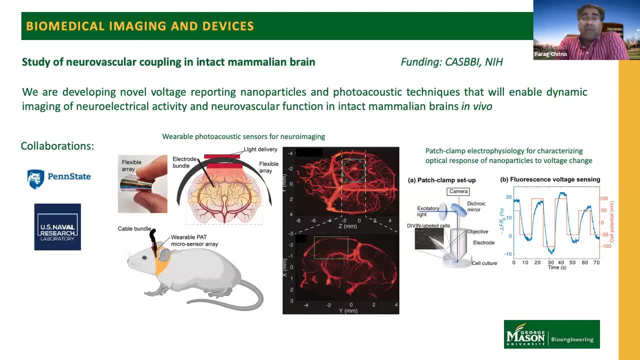 through tissue better. So together we get the military sound and the ultrasound can penetrate through tissue better. So together we get the military sound and the ultrasound can penetrate through tissue better. So together we get the military specificity, but at deeper locations and tissue. So this could be useful for studying the brain. 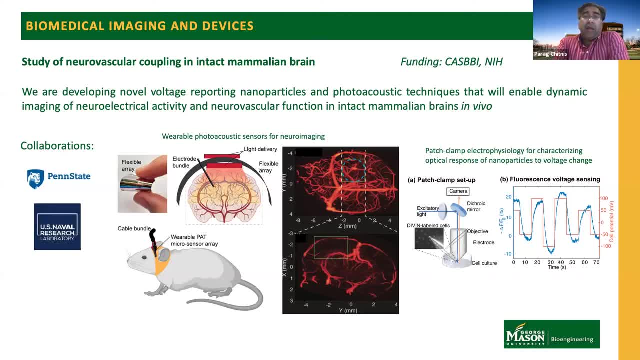 through intact brain tissue and skull. Photoacoustics have already been established as a very good imaging modality for looking at blood and hemodynamic function. So in our lab we are collaborating with nanoparticle experts to develop voltage reporters that can be. 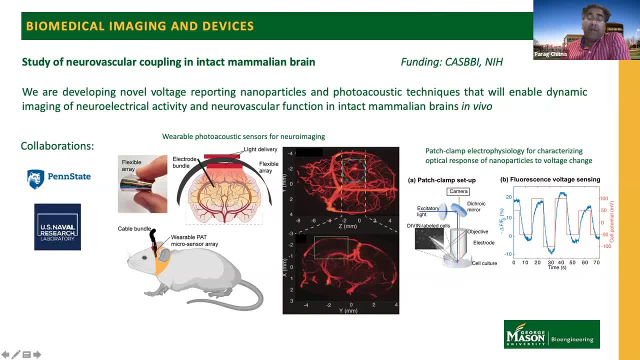 that can give us a voltage readout. For example, here we have combined a power clamp and a fluorescence microscope to test how well the nanoparticles that we have developed work for giving us a voltage readout. As you can see here when the voltage has been modulated of 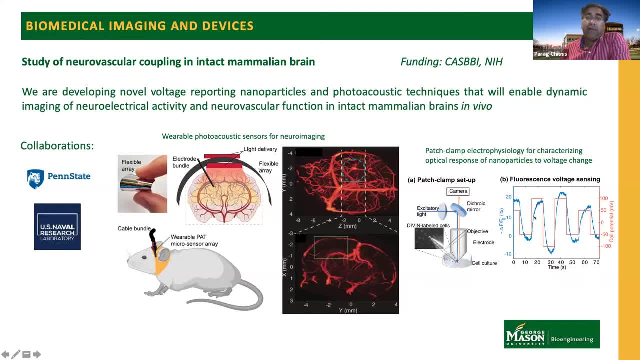 a cell membrane, we can see that the optical readout from those nanoparticles also modulates along the same way. Now we are also developing in silico simulations to design photoacoustic sensor arrays that would give us good imaging in the mouse brain, And we're collaborating with 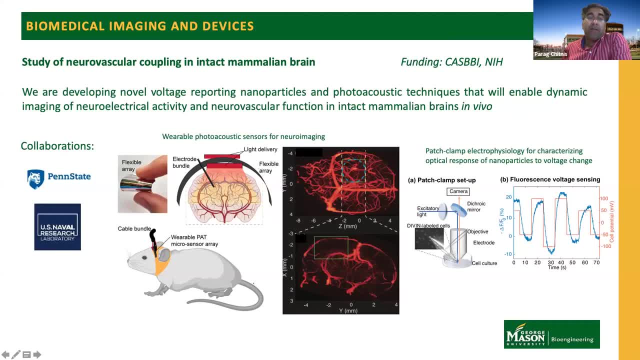 experts at Penn State to develop flexible photoacoustic sensors that can be mounted on the animal so we could perform these studies and they awaken behavior. Long-term goal of this work is to develop a toolkit that can be used to answer several pertinent neuroscience questions. 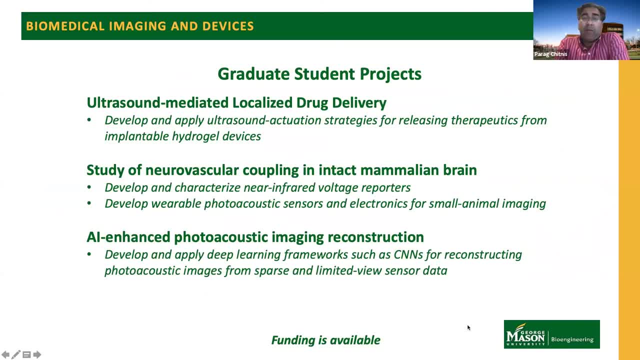 So both of the projects that I described today have openings for better students, and students from a variety of backgrounds can come and work with us, including biologists, chemistry, instrumentation, signal processing. In addition to those two projects that I described, a third active area of research in my lab involves machine learning- artificial intelligence for 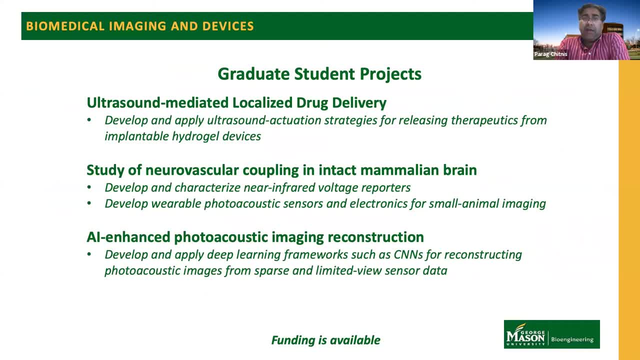 photoacoustic imaging reconstruction. Specifically, we are developing deep learning methods, such as convolutional neural networks that are optimized for imaging the mouse brain, especially when the data is acquired from sensors that suffer from sparsity or limited view. Funding is available for all of these projects and we are working with the University of Michigan at the University of 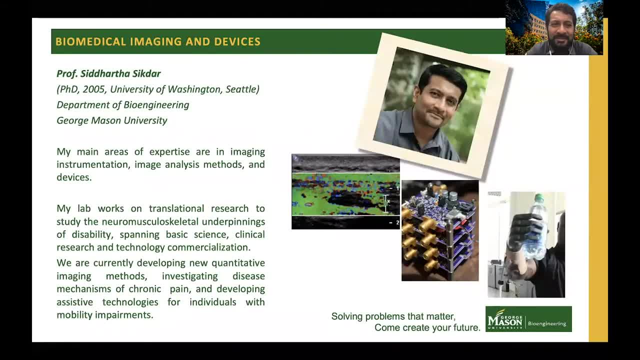 Michigan, as a full-time research group in Echo Valley. We are working on the next few weeks and we look forward to hearing from you. Hello, my name is Siddhartha Sekadar. I'm a professor in the Biomedical Imaging and Devices Pillar. My main area of expertise is imaging. 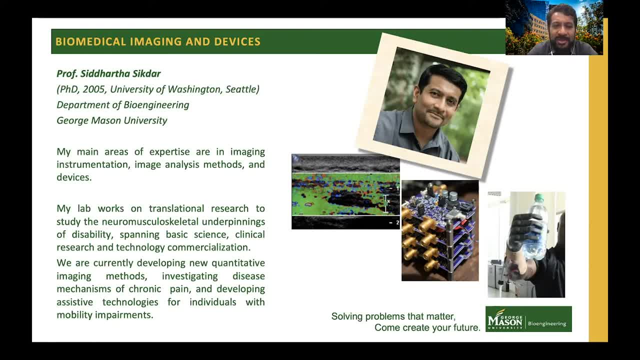 all the way from image analysis methods to image instrumentation and devices. My lab works on translational research to study the neuromusculoskeletal underpinnings of disability, and our research spans both scientific clinical research as well as technology commercialization. 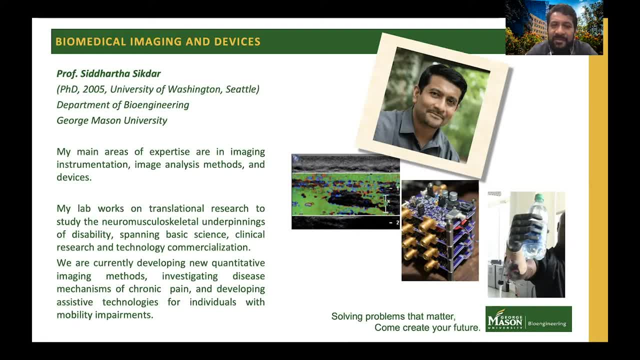 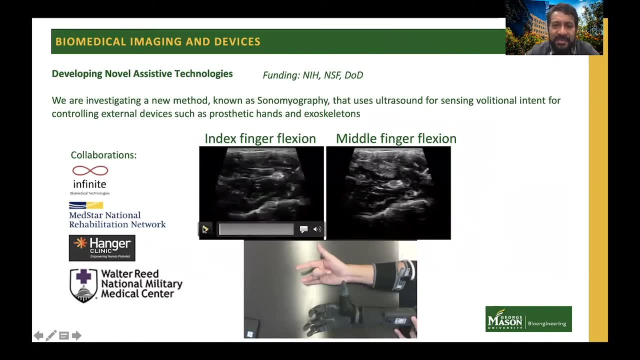 We are currently developing new quantitative imaging methods and allows us to get more methods investigating disease mechanisms of chronic pain, as well as developing assistive technologies for individuals with mobility impairment. So I would like to highlight one project in my lab. This is a project that is funded by the National Institutes. 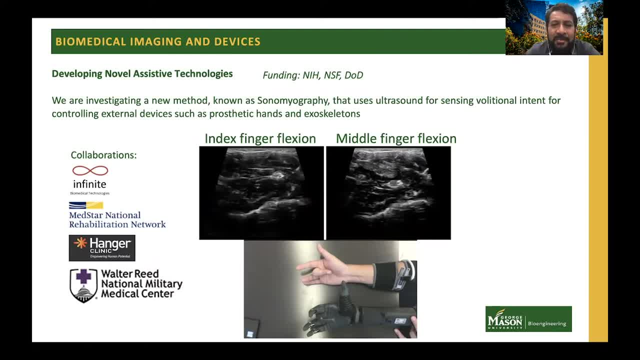 of Health, National Science Foundation, as well as the DoD, And the idea for the project is to develop the next generation of prosthetic control devices. So in the field of prosthetic control, surface electromyography has been the predominant method for sensing muscle activity and inferring. 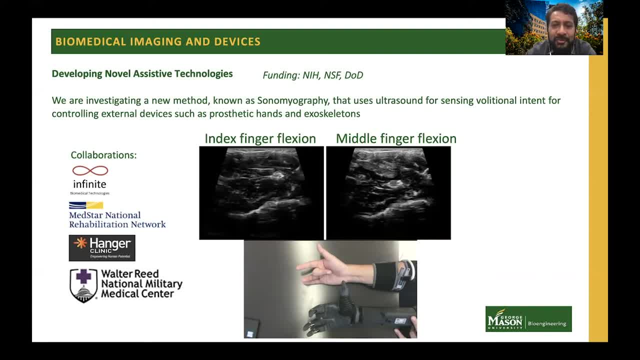 the volitional intent of users who have lost limbs. There are well-known limitations with electromyography, including poor signal to noise, the inability to differentiate between muscles that are deeply embedded inside the tissue. So in my lab we have been using a new method. 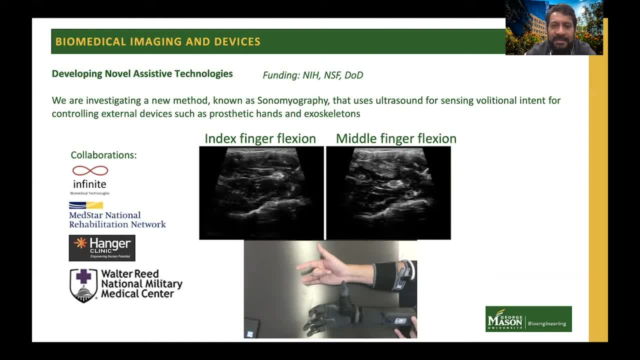 known as sonomyography, that uses ultrasound for sensing muscle activity, And this method is very similar to that of prosthetic control devices, But it's a little bit different in that it's using the volitional intent, And so the idea for sonomyography is. 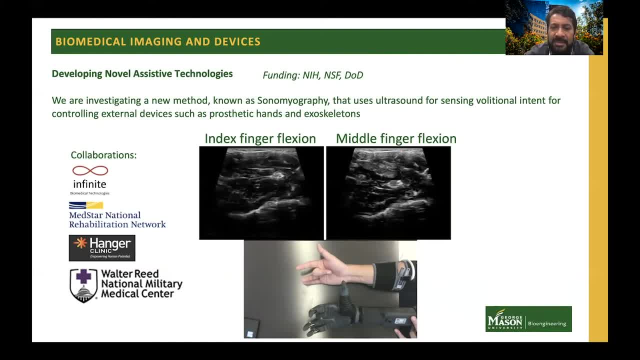 that we image the cross-section of the forearm using ultrasound And we can actually infer the intent from the patterns of muscle activity. So when a subject is trying to do an index finger flexion, we see a particular muscle group that's activated when the same subject does a middle finger flexion. 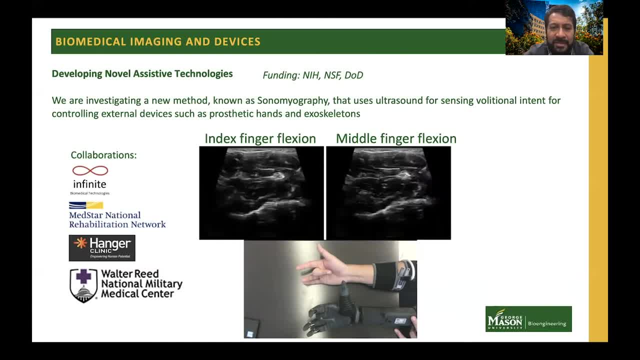 a completely different muscle group gets activated, And so we can see that there's a difference between these two types of image sequences and then use that to control a prosthetic device. So, for example, here is a user who is controlling this prosthetic hand based on the signals. 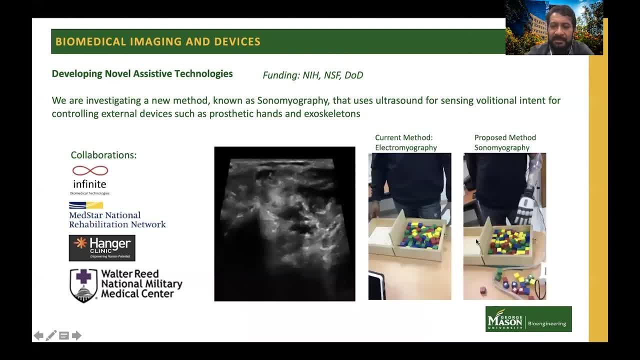 that we are getting from the muscles. So we are currently testing this in amputee subjects, So we can similarly record ultrasound images from the residual forearm of these subjects And we are testing whether they are able to compare against conventional electromyography. 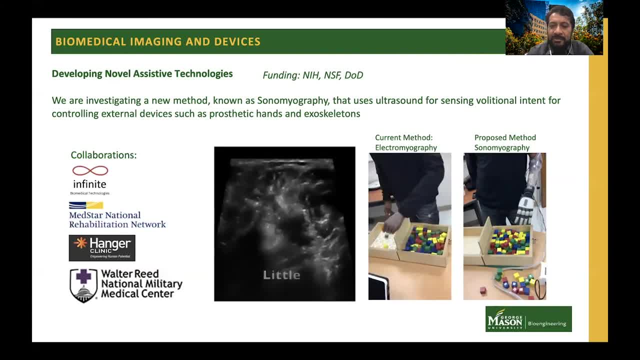 So there is one case where the user is trying to use conventional electromyography based prosthetic hand And you can see that he's struggling to pick up these blocks, And so he's compensating using his trunk as well as other compensating movements. 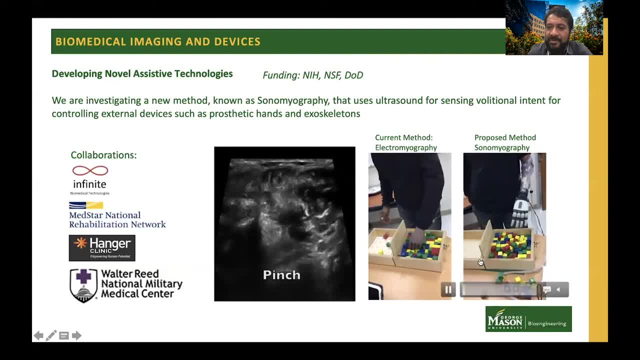 If the same subject is now instrumented with an ultrasound transducer to sense the muscle activity while they're imagining these movements, you can see that they are having better control over their terminal device. So they are standing up straighter, not using as many compensated movements. 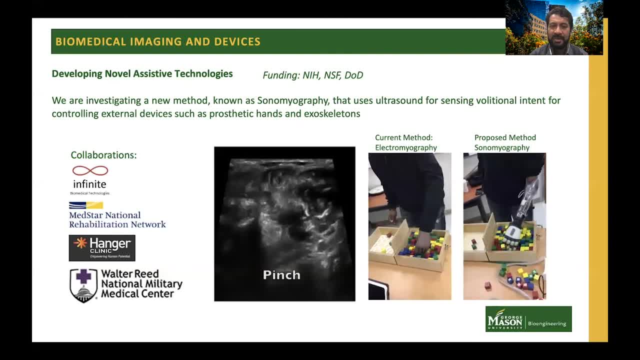 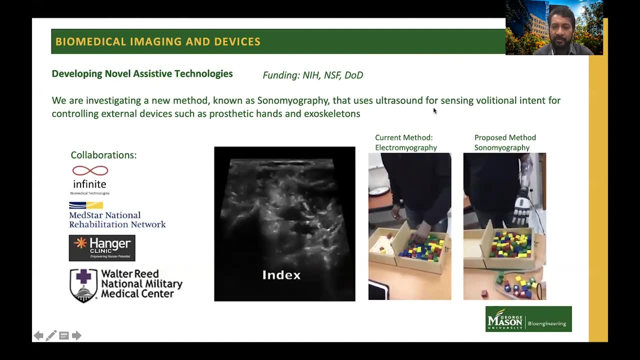 So this is an ongoing project that is being done in collaboration with industry partners- infrared biomedical technologies. We are also working with a number of clinical partners, including MedStar National Rehab Hospital, Hanger Clinic and Walter Reed National Medical Center. We have a number of open positions. in our lab for graduate student projects And if you can find a candidate by any chance to contact us, you can contact us. If not, you can contact us right now. Thank you, Thank you very much. Thank you, Sir, Thank you. 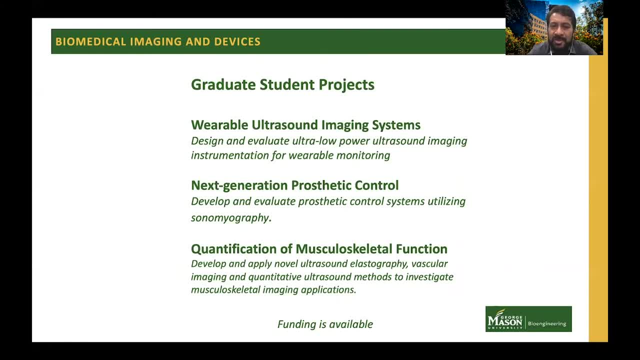 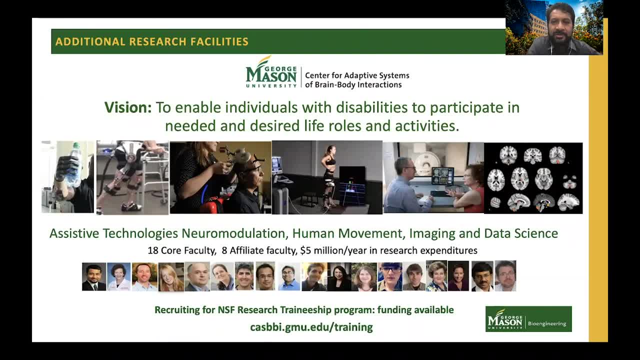 In addition to my role in the Department of Bioengineering, I'm also the director for the Center for Adaptive Systems of Brain-Body Interactions. This is a transdisciplinary center at the university with a vision to enable individuals with disabilities to participate in needed and desired life roles and activities. 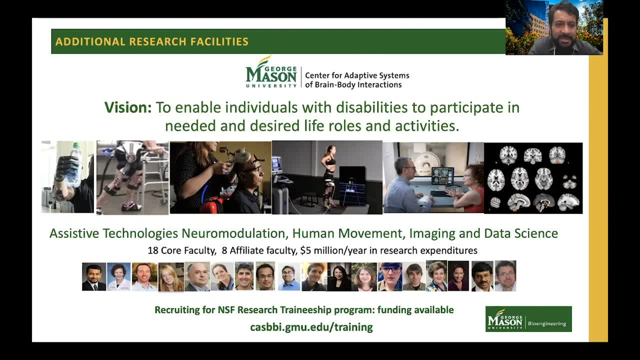 At the center. we have a number of state-of-the-art facilities for developing assistive technologies, for neuromodulation, for studying human movement, as well as multi-scale imaging, all the way from small animals all the way to humans. We have a number of faculty in the center who have broad disciplines.